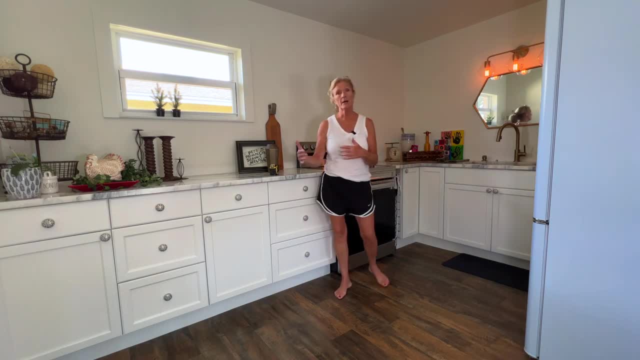 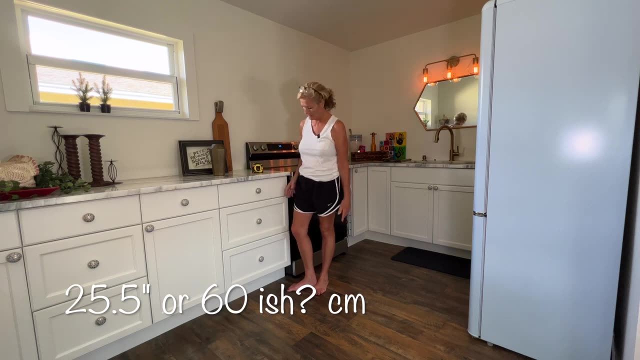 See inside the cabinet. They- they're a little bit shy of that. They're about 18 inches deep. The countertop itself will extend out to 25 and a half inches. That's because you have the drawer faces, So you have 24 inches for. 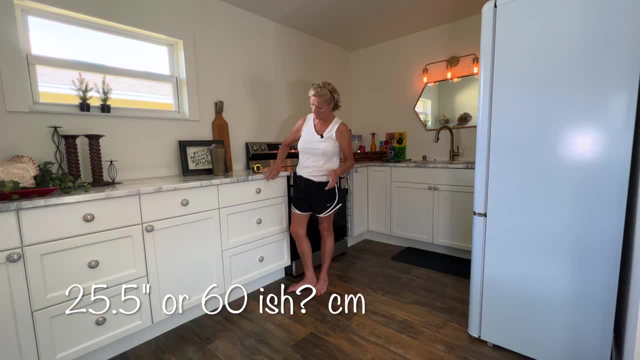 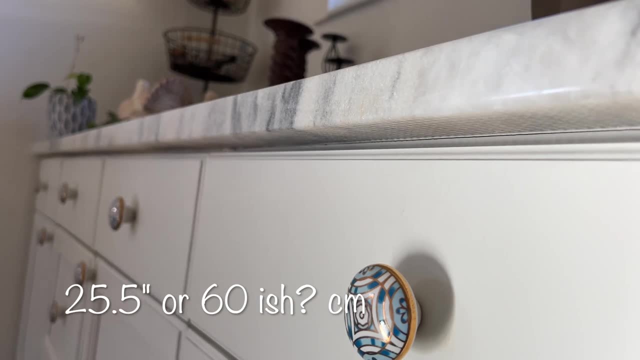 the box, another three quarters of an inch for the drawer face, And then the countertop itself hangs over another, sometimes an inch, sometimes three quarters of an inch. That's really up to you and your fabricator The reason for that, and I've seen a lot of people asking for this lately- 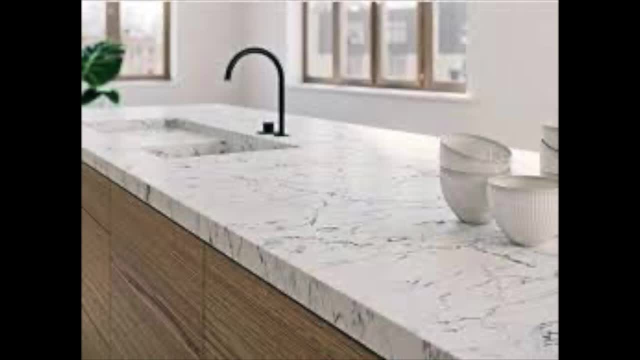 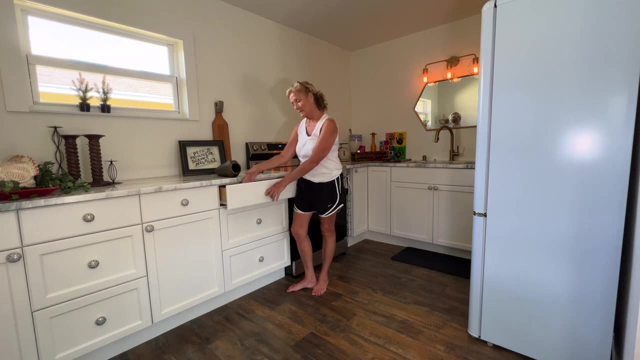 is that it's a drawer, So you have the drawer faces and the countertop flush And that's marvelous. It looks so cool, But if you've got kids and they spill something, it's going to sit in here Or, worse, it's going to get inside each of these drawers every time. The reason this? 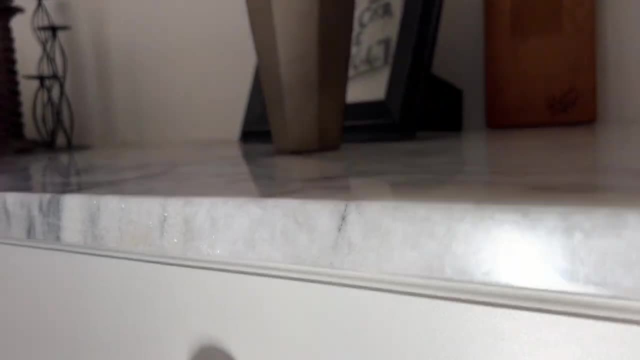 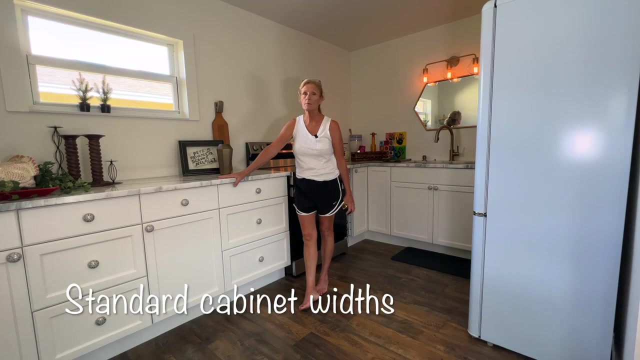 overhang is here is so that anything that spills is not going to hit the face of your cabinets. Keep them clean. So that's up to you and your tidiness and your family. I know for me we have an overhang. I've seen three inch, which are completely useless, Six inch, which is really stretching. 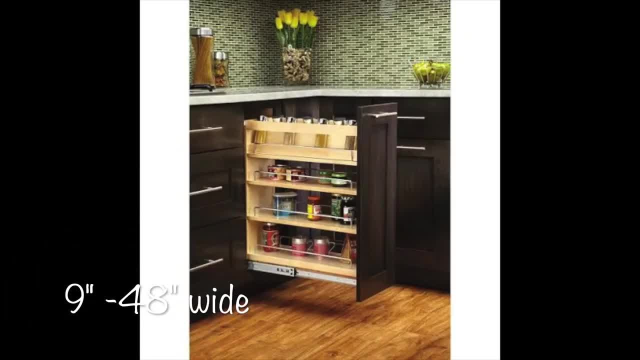 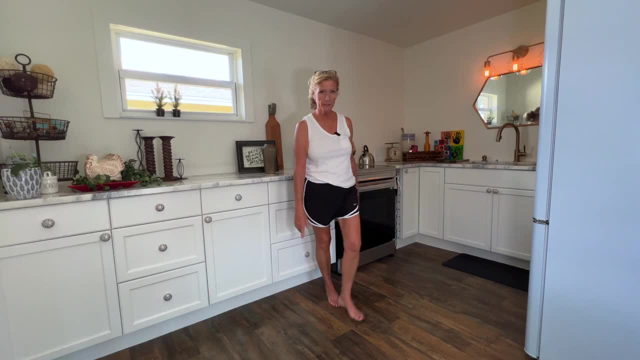 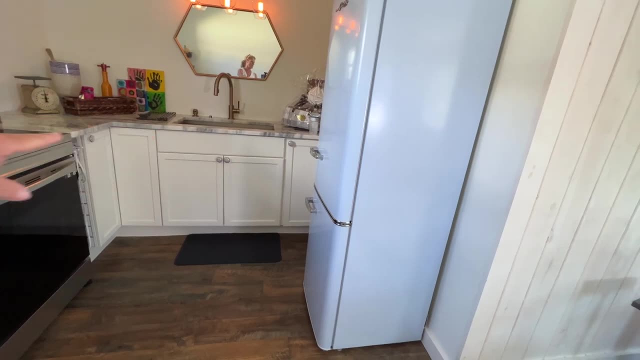 on the usefulness And the nine inch pullouts with your spices, and all of that On up to 48 inches for corner cabinets. We have a 36 inch cabinet here. Let's see if I can switch you around. There's our 36 inch cabinet there And that's got two knobs, So anything over 24 inches wide. 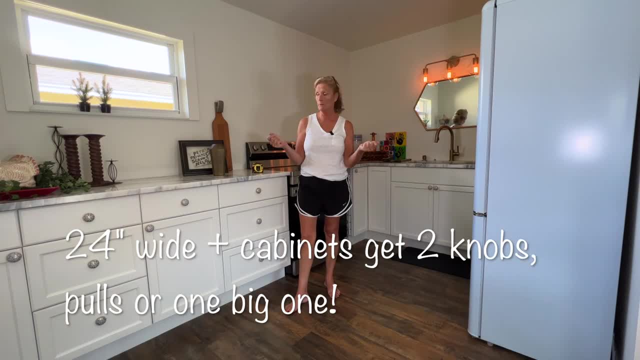 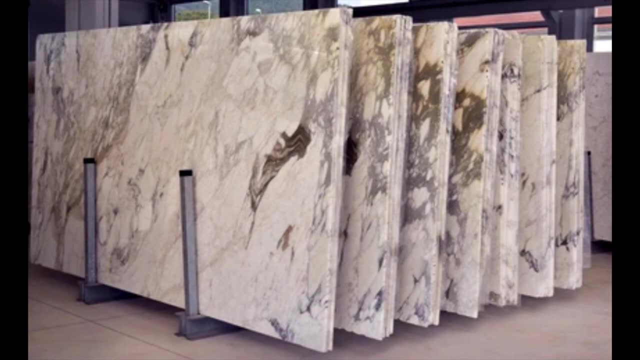 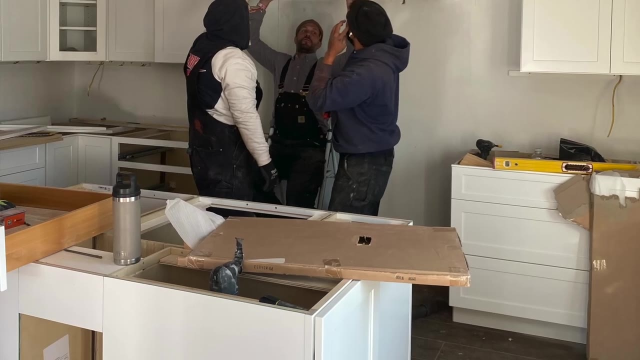 needs two doors And two knobs, two handles or one big long handle. When it comes to the island, it's just a bunch of base cabinets with a countertop thrown on top and some end panels or finished panels to wrap it out. You need to support the countertop, So a lot of times you'll 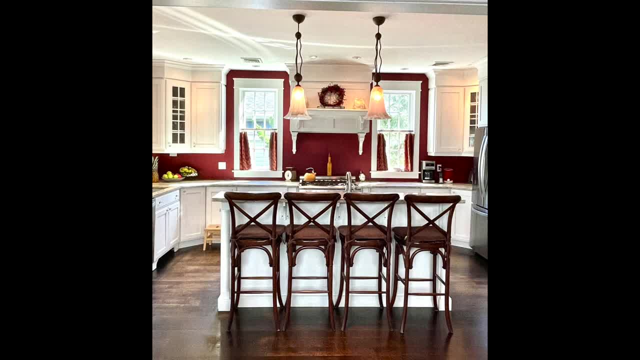 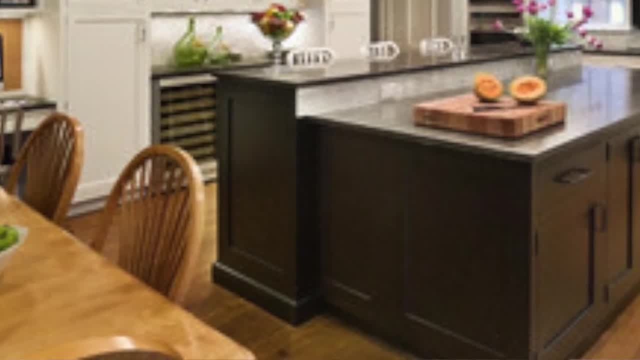 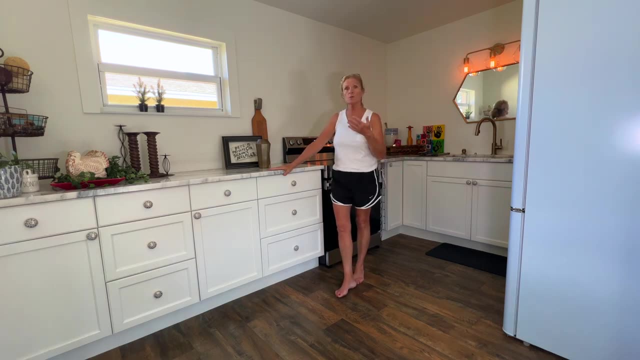 use cabinets all the way around. If you have a two tier height island, you can use a base cabinet for one side and a wall cabinet at 42 inches to support the countertop. at a higher level, You can also use 18 inch base cabinets or 12 inch base cabinets to support the island. 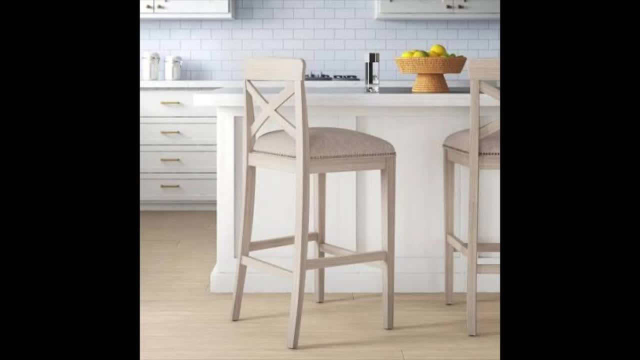 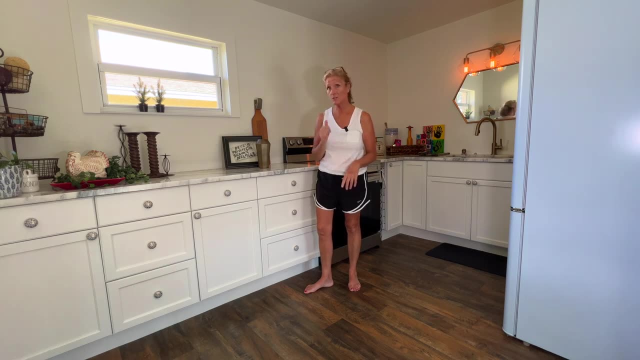 and have 12 inches or 15 inches for the overhang that you need for your leg room. If you have any questions about the measurements regarding an island, I have a video about it. Go back and watch it. It's a good one. We don't have any uppers in here And we really don't have 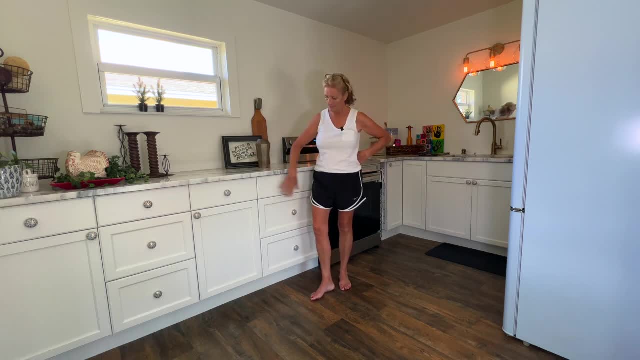 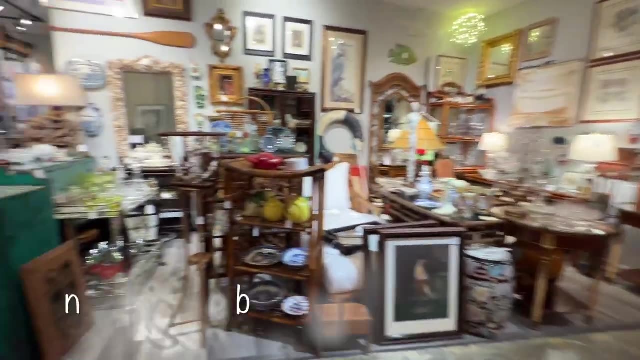 a need at this point because it's a pool house, So it's got enough storage. However, I've been eyeing up a pair of vintage corner cabinets that I think would be perfect for this island. I've been that match the theme in here, with sort of the diamond shape She's been holding. 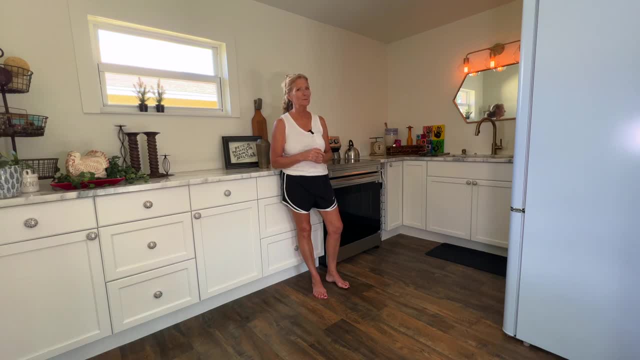 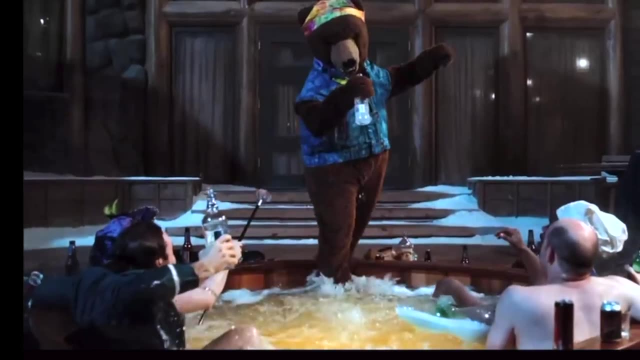 on to them and hasn't lowered the price yet. but they haven't gone yet, so I'm keeping my eyes peeled for that. Now we have to go back to the 90s to see about the uppers, And we're in the 90s. 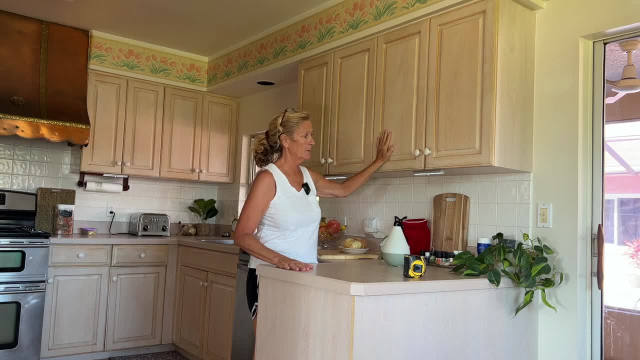 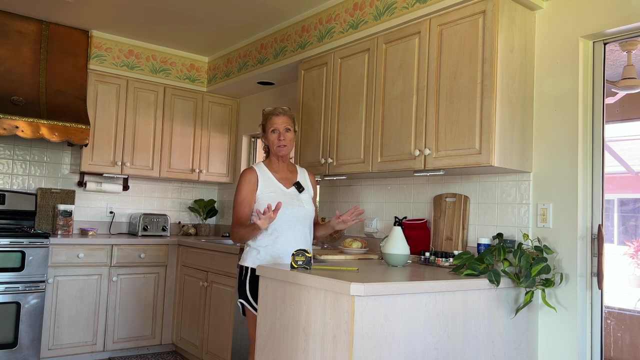 Hot tub time machine. These upper cabinets are 12 inches deep, so 12 inches off the wall. The reason for that is when I stand here I don't want the cabinets to hit me in the face. Upper cabinets come much the same as lowers, as far as the sizes go, Every three inch increments. 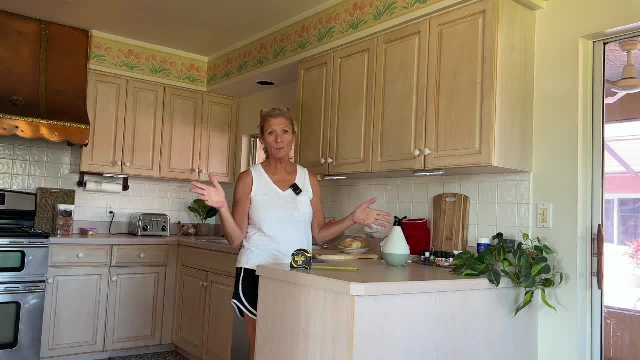 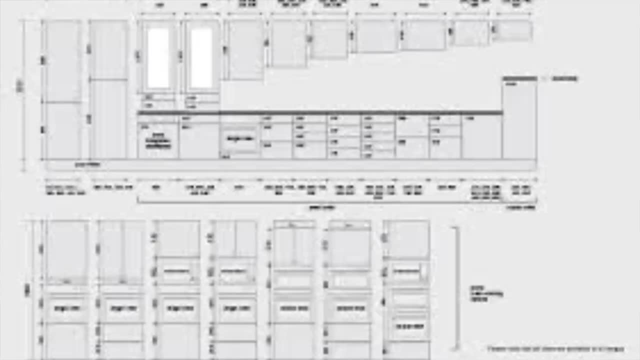 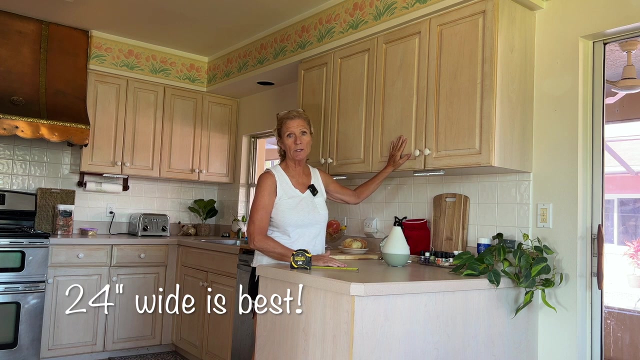 so if you can stay 15,, 18,, 21,, 24, you get the idea. If you can stay within standard stock sizes, you can save yourself a lot of money when you're planning a kitchen. From a six or a nine inch cabinet on up to probably a 36 is as wide as you want to go. 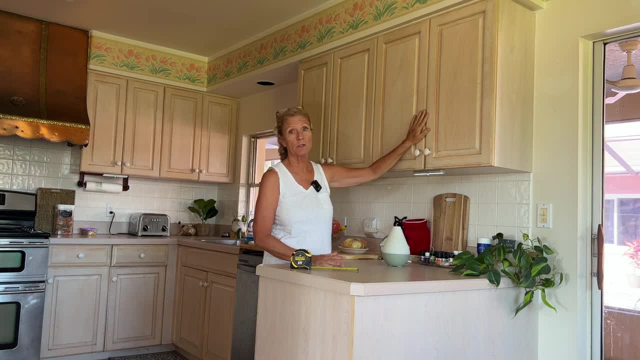 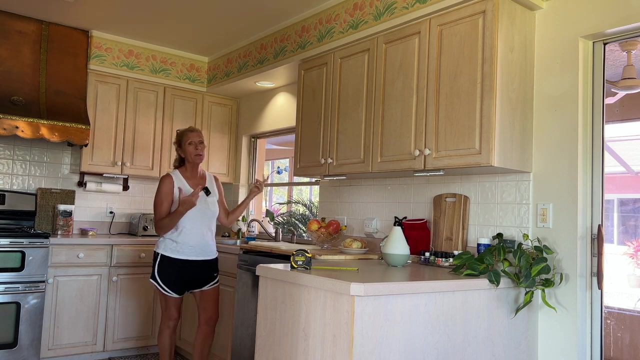 For uppers. there's a couple of reasons for that, and this is a good example right here. This is a 30 inch upper in an eight foot ceiling with the hideous soffit from the 90s. There's nothing up there. They happen to run some light over here, which is over the sink, which is nice, but the 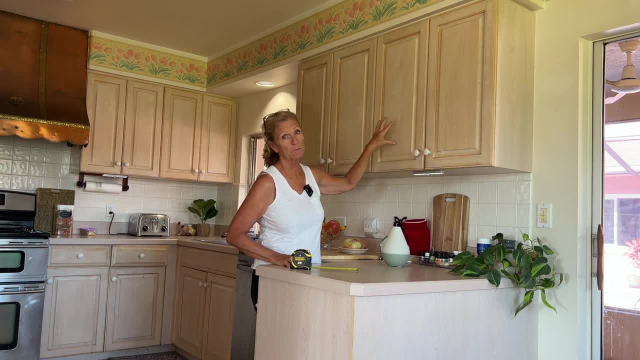 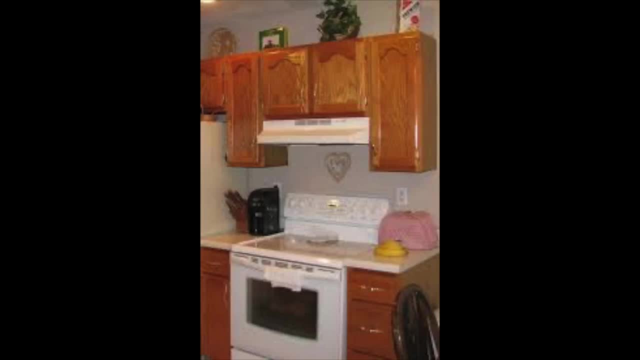 soffit was very popular to do because it allowed you to get the less expensive cabinets and not have that dust collector up there or just this random space at the top of the cabinet, And I really like that. I think it's a great idea. I think it's a great idea. I think it's a great idea. 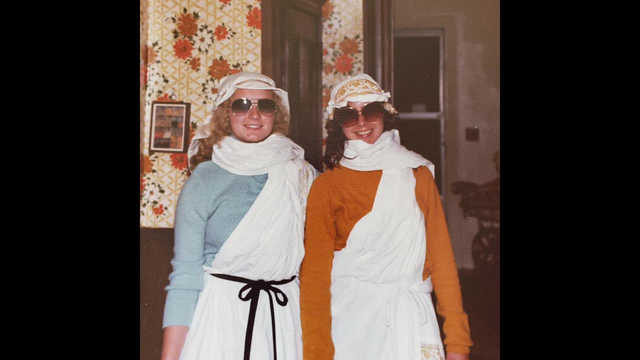 And I really like that. I think it's a great idea. I think it's a great idea. I think it's a great idea. I will tell you, having cleaned beach houses for many years with my best friend, Chrissy- nobody goes up there and cleans that. I have a pantry over here and I can guarantee I haven't. 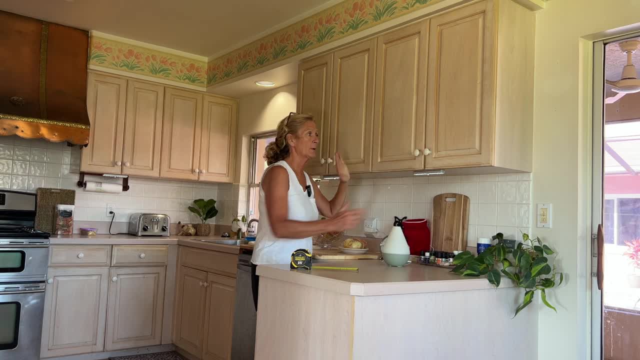 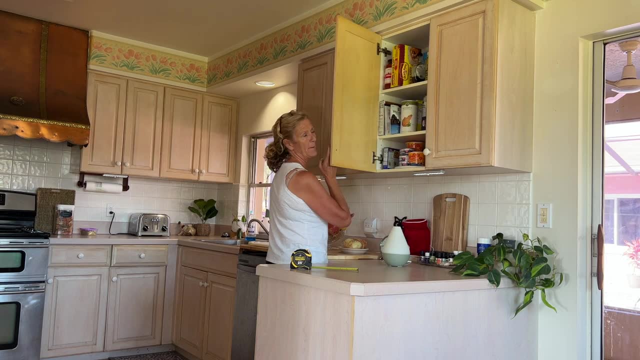 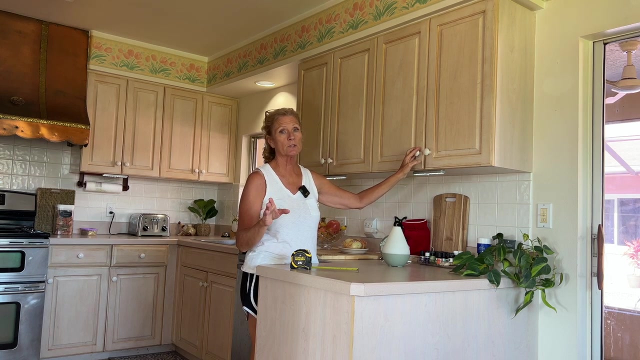 been up there, I could do without it. So these are 12 inches deep and this particular cabinet is 30 inches wide. It's got a 15 inch door here And if I'm standing here, bam, bam, bam right in the face. Now I said, with base cabinets, anything over 24 inches is going to have two doors. 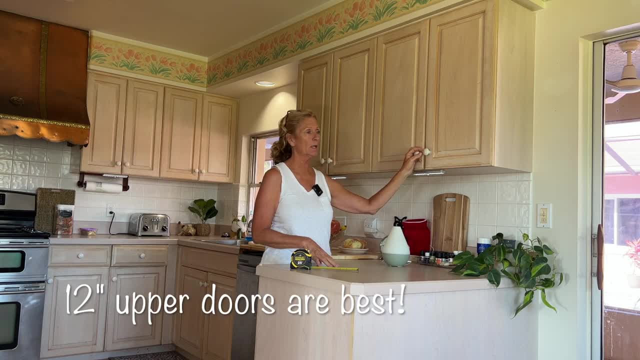 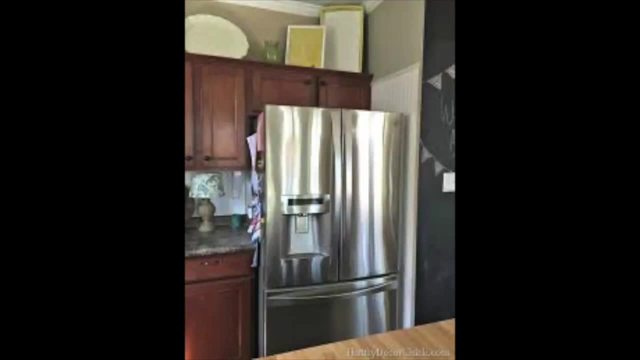 But when it comes to uppers, you want to keep the doors to 12 inches, if you can. 36 inch cabinets are going to give you an 18 inch door. You're going to have to step way back in order to open it. You can get uppers from 12 inches high. 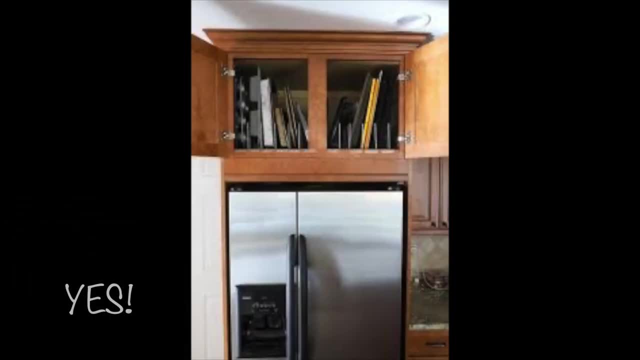 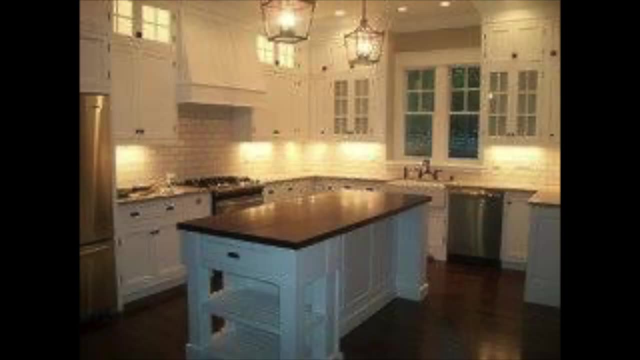 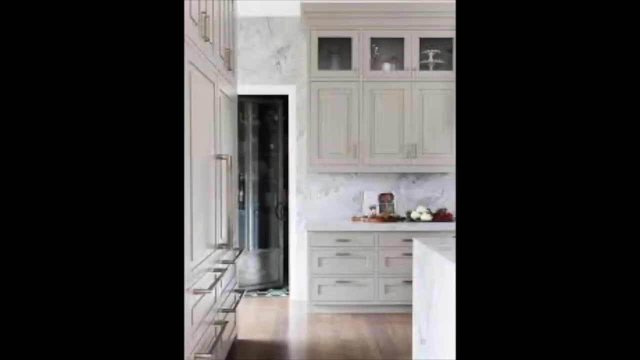 that go over a fridge to 24 up to 54 inches high. You can also stack boxes on top of each other. However, I would caution you when you're thinking about this. I have a lot of clients that want to do this And basically you're buying two kitchens and you're not getting the function of it. 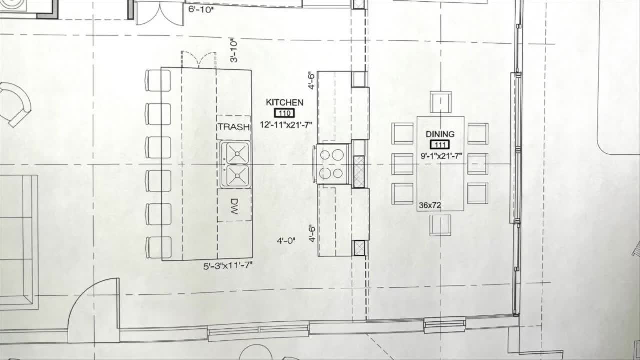 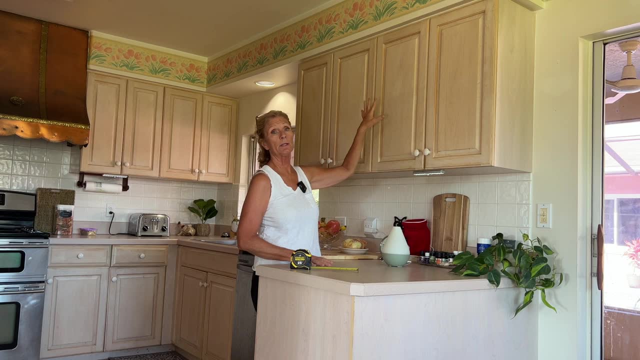 You're buying two kitchens, because kitchen cabinets are charged by the box and then they mark it up for the size and for all the extras inside. So if I have an upper and I put another cabinet above it, let's say I have 10 foot ceilings and I do a 42 inch closed cabinet. 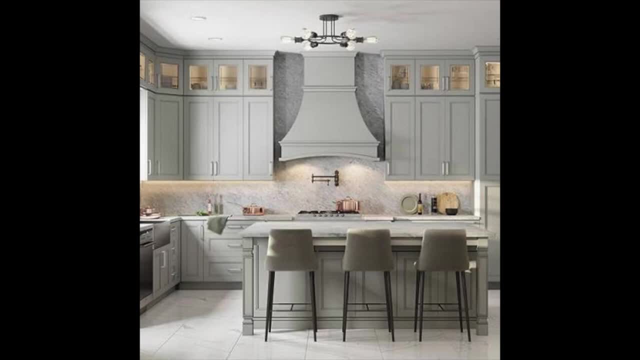 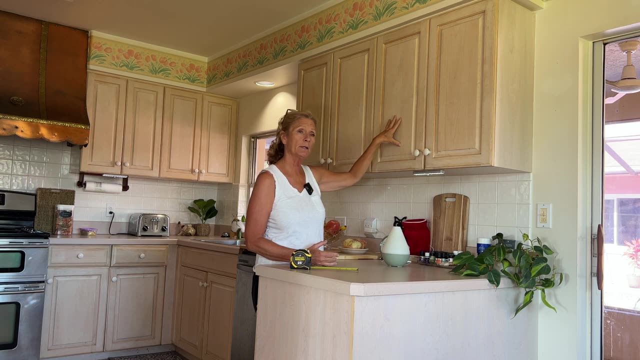 with an 18 inch cabinet with glass doors and a light above it. that 18 inch cabinet is going to cost the same or more, with the glass and the light, than this cabinet here. So when costs are an issue, go to the ceiling with one box, And there's a couple of ways you can do that without the 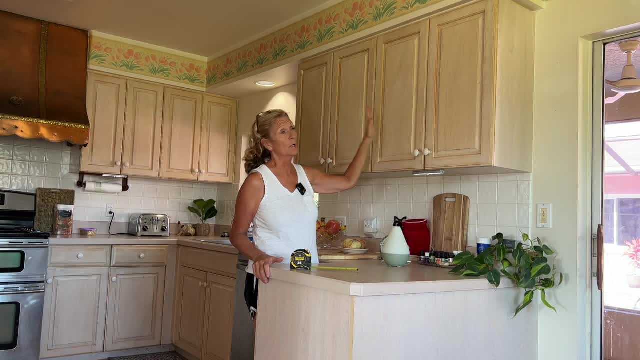 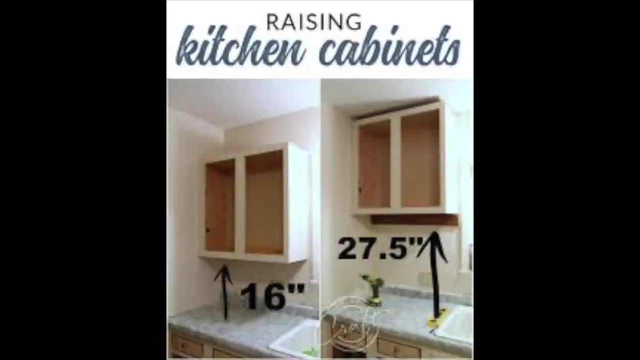 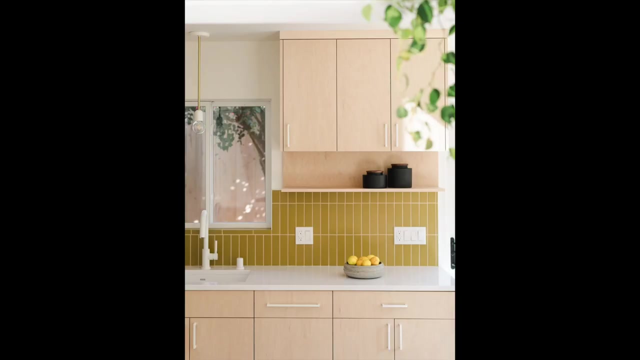 dreaded soffit. If budget is an issue and you don't want the soffit and you don't want the empty space, the smartest solution I've seen is to raise the 30 inch cabinet or 33 inch cabinet to the ceiling and to do an open shelf below And that gives you the best of both worlds. I know that. 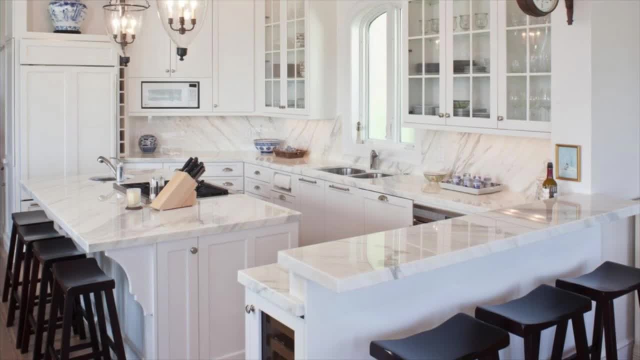 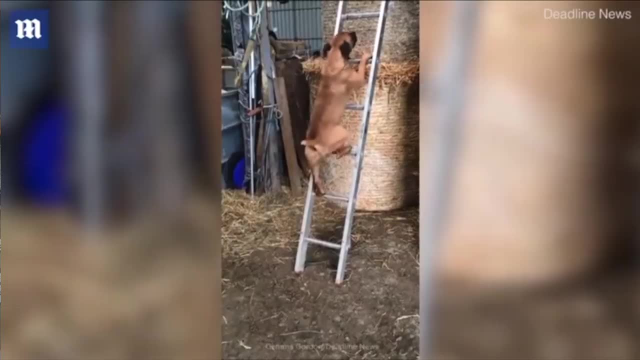 when you're doing a kitchen, you get excited and you want to fill the space with cabinetry. But when it comes to upper cabinets, you want to fill the space with cabinetry And when it comes to cabinets, anything beyond the second shelf- for me at 5'6- is useless without a stool. The trend has. 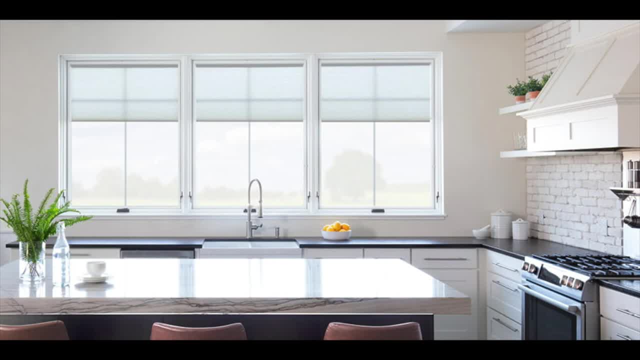 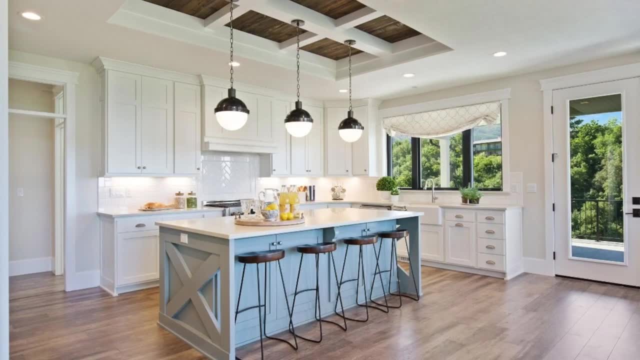 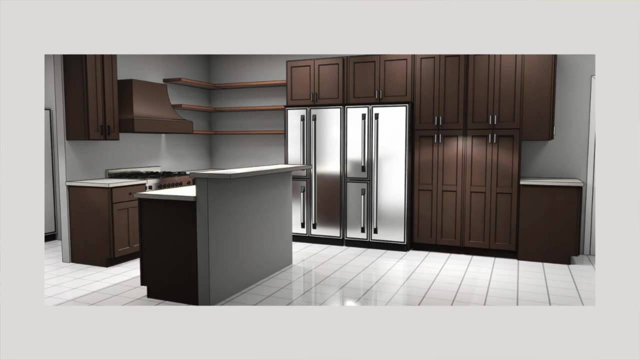 been to do less uppers because really, when you think about it, glasses, a few items, mugs, those are the only things that really need to go in an upper. It can save you money. it can open up the space by not having so many boxes Because, again, cabinet makers charge by the box. first, A thousand. 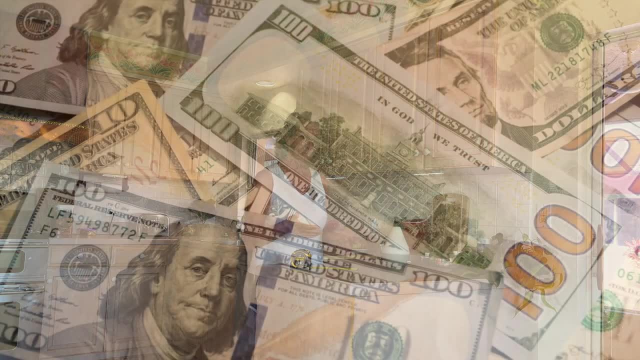 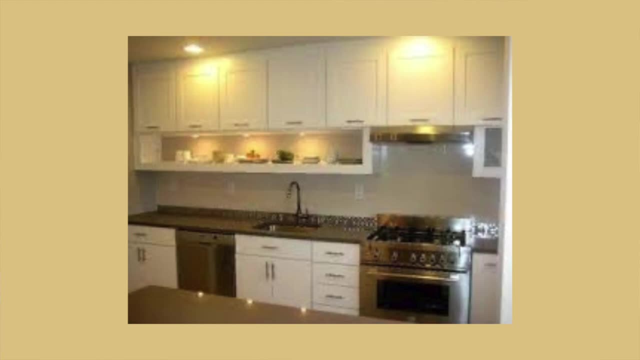 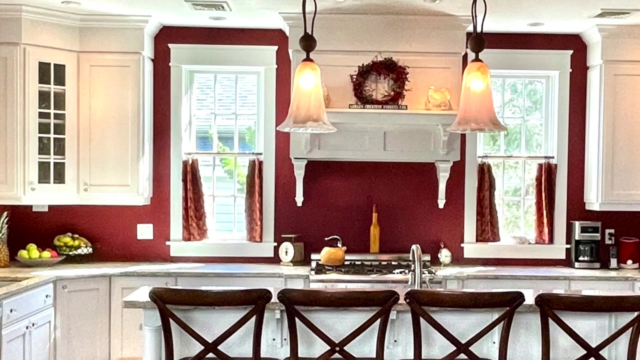 dollars for each box, you can start to get an idea. If you don't want to raise your cabinets up to the ceiling and have an open shelf, the thing that I did in my kitchen with nine foot ceilings is I had 42 inch uppers and I had what's called a fascia. 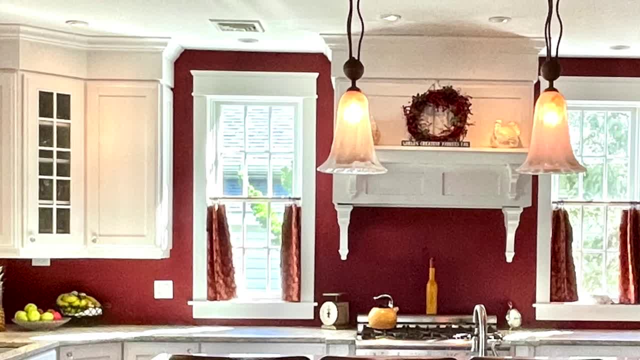 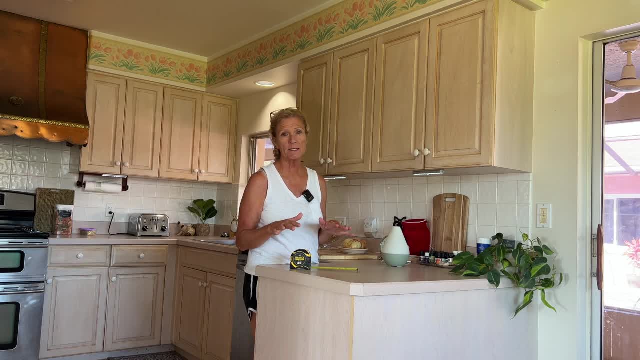 board or a flat piece of stock wood and then crown molding. And this is great because no ceiling is perfect. You got a better shot with older houses because they've already settled Piece of wood. you can get it from your cabinet maker to match and it just runs the length. 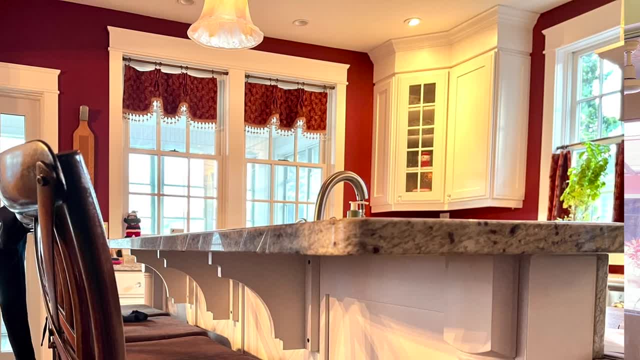 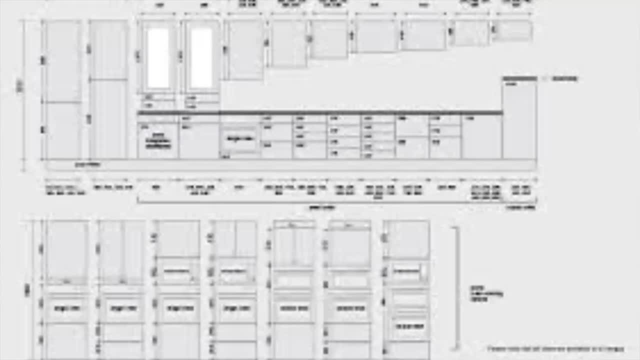 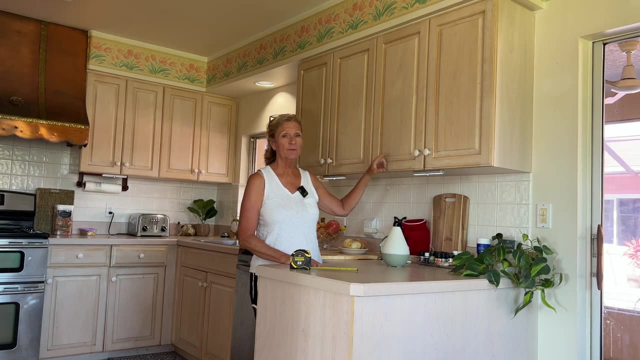 And then you put a piece of crown at the top and it finishes the cabinetry all the way to the ceiling. It's a much nicer look than leaving that space empty or doing a stopper. The standard measurement for uppers is 42 inches above the finished floor or 18 inches above the countertop. However, if you 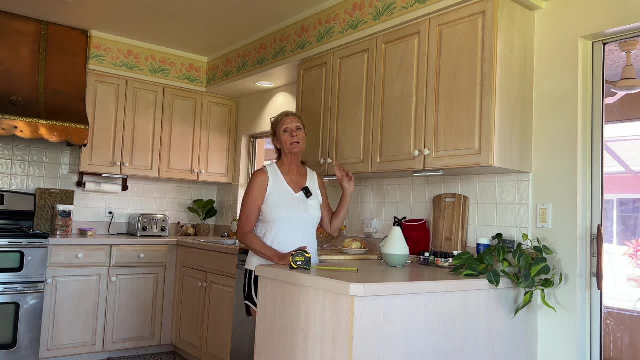 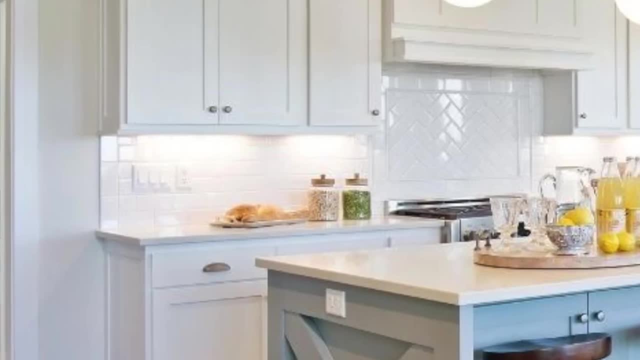 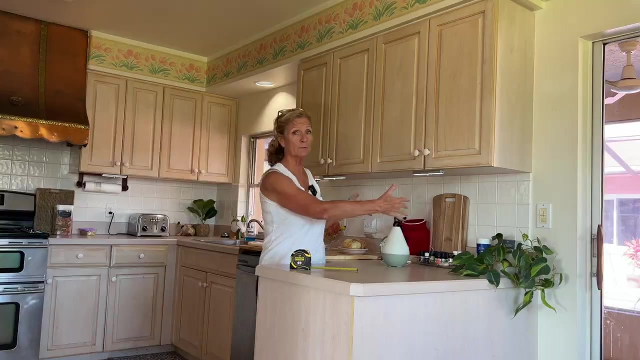 have the room push it up to 20 or 22,, especially if you're going to add under cabinet lighting and a light rail or piece of trim along here that's an inch or two inches thick, so that it doesn't slide in Things like my Vitamix or a Redhold espresso maker. they won't fit underneath. or 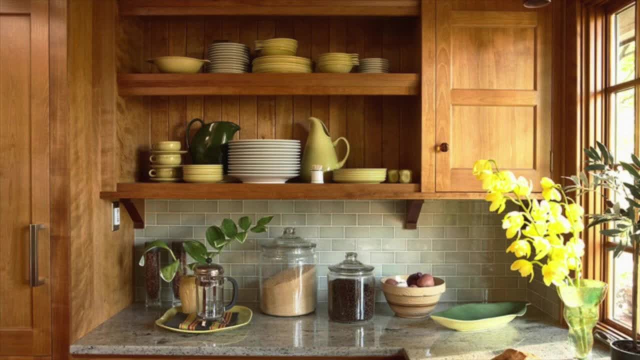 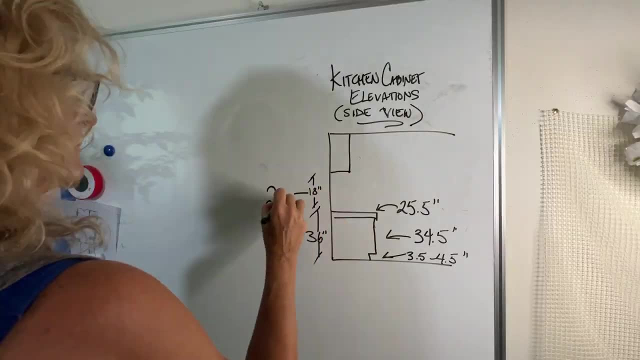 you won't be able to access the top of them if you lower this down. So 18 is kind of tight. If you've got the room, push it up. 20,, 22 is really nice. Last up in the cabinetry is pantries and we all. 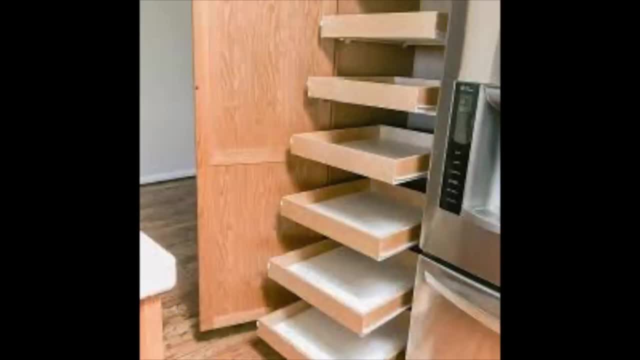 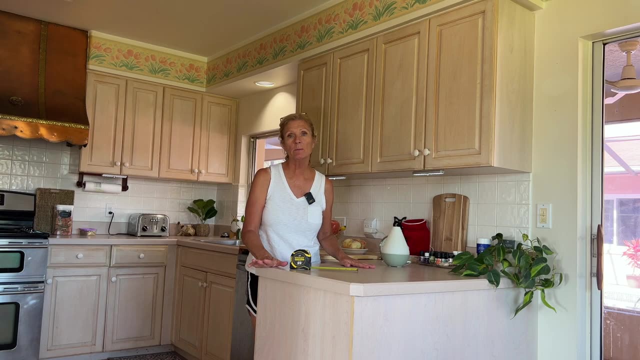 love a good pull-out pantry. Most of them from your cabinet maker are going to be 24 inches deep. They do have 18, some even larger. We're going to offer a 12-inch pantry. There's two things you want to keep in mind with the pantry. 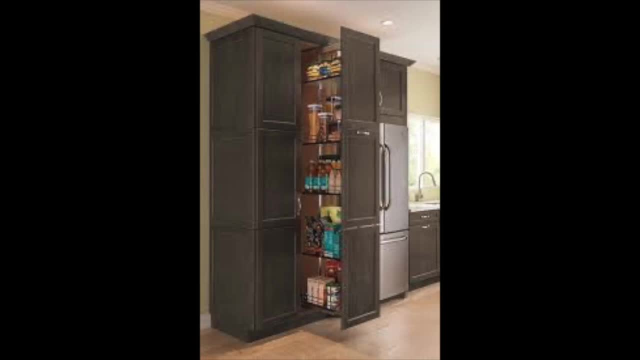 First of all, the stuff you're going to be putting on. it is heavy. I know we want a really big cabinet to put a lot of stuff on, but if you've got pullouts on there and you're putting a case of water or 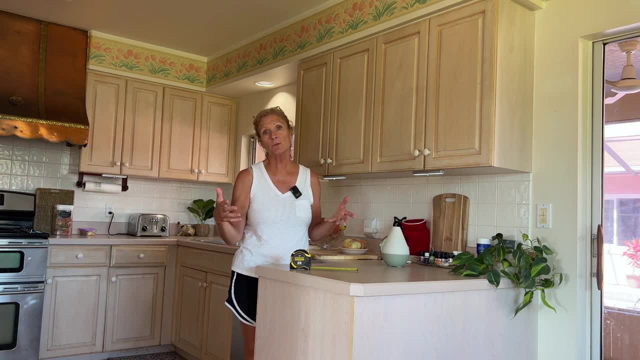 heavy canned items. that over time is going to make those drawer slides fail. 24 inches- 18 inches- is a nice sized pantry. This isn't really for your Costco BJ's bulk items. This is for your dry goods, for your everyday items. If you've got a really